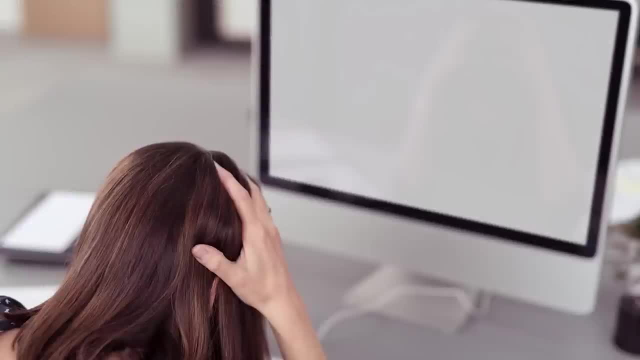 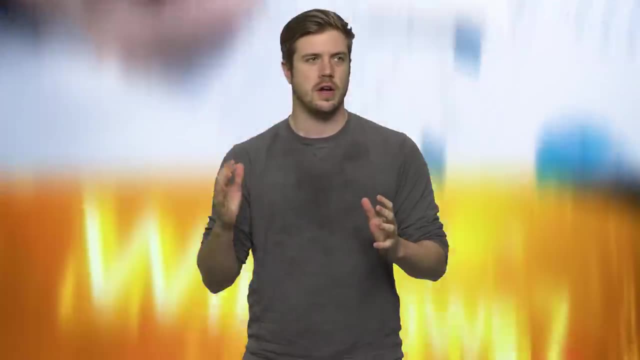 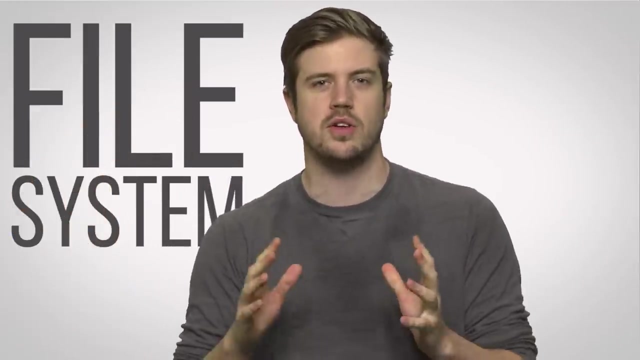 done that, But anyways, could you imagine if your computer was that forgetful and never remembered where you put stuff like save games, important papers or tax documents or your operating system? Fortunately, all computers use some kind of file system so it can keep track of where all your 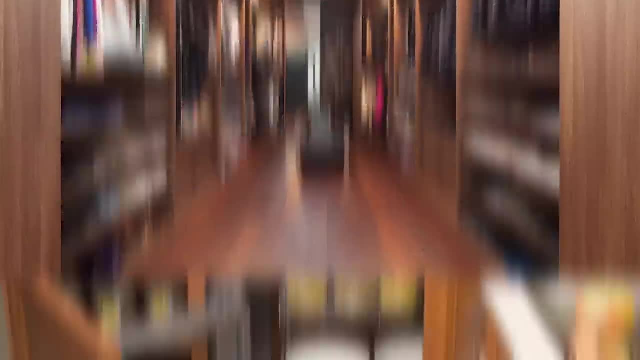 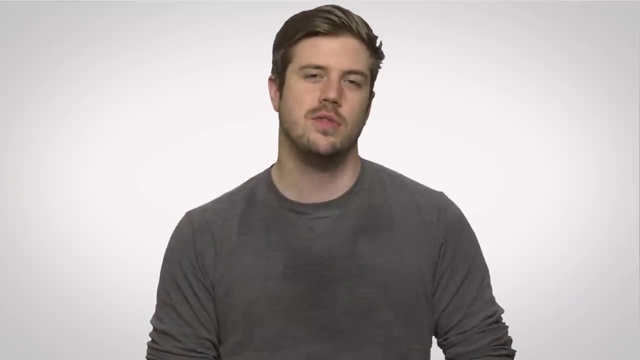 stuff is Just like how you might use a closet space or cabinets at home to keep your collection of random clothes and kitchen items from being a complete mess. So how do they do that? Well, there are many different types of systems out there, but what they all have in common 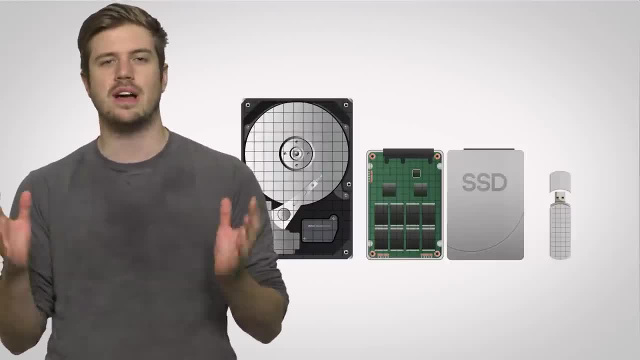 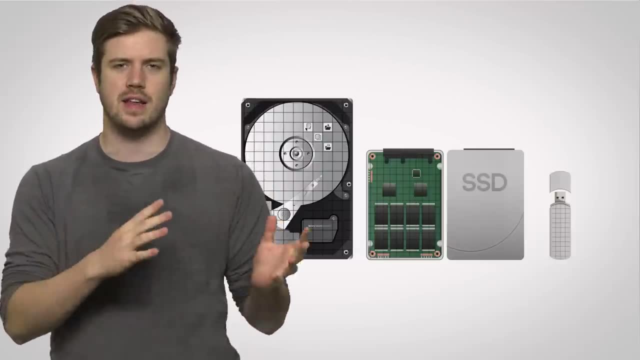 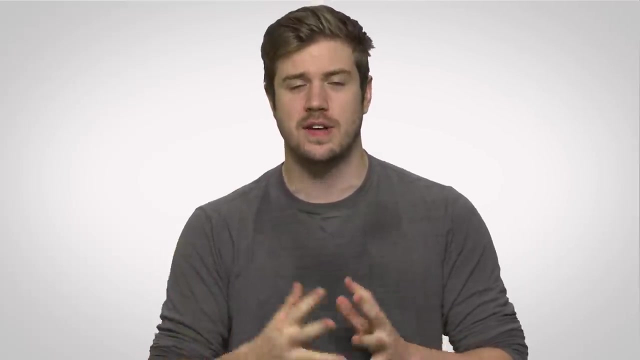 is that they divide up your hard drive, SSD or flash drive into small units that store data and have some kind of way of remembering what data is in each unit so it can go and find it later on. To better understand how this works and to figure out what system to use for your own stuff, let's have a look at some common file. 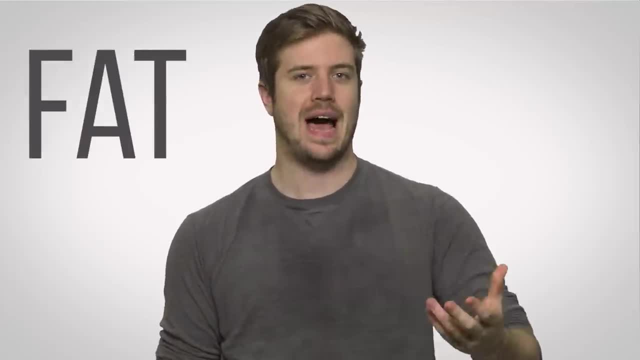 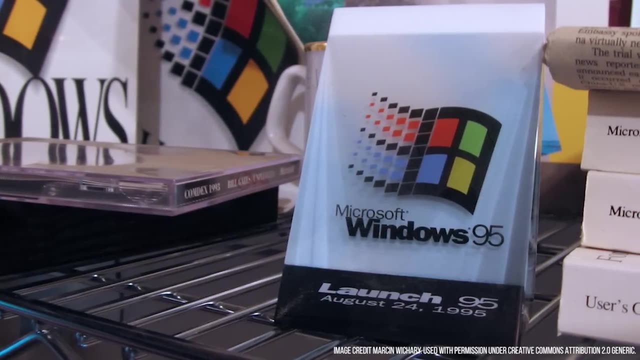 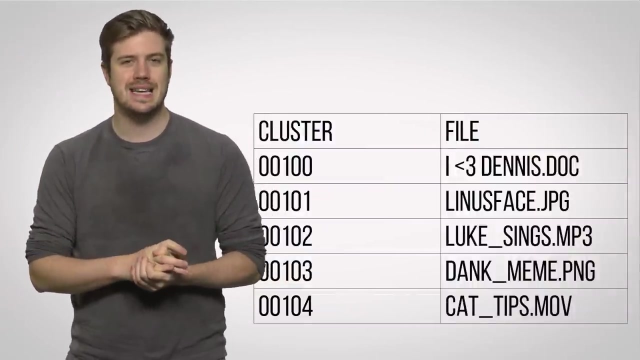 systems, starting off with File Allocation Table or FAT, And although its name is incredibly unflattering, FAT was used by the vast majority of home Windows-based PCs until XP came out. FAT worked by splitting the disk into a bunch of clusters, giving each cluster a unique ID number. 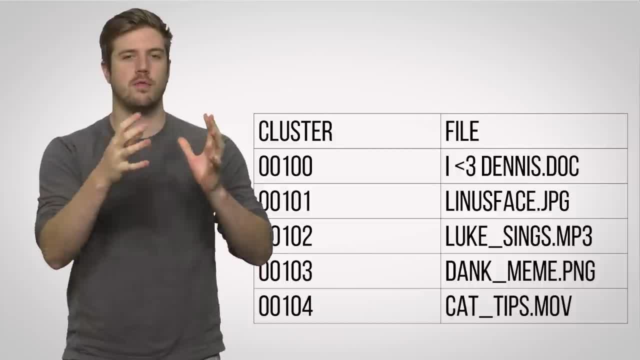 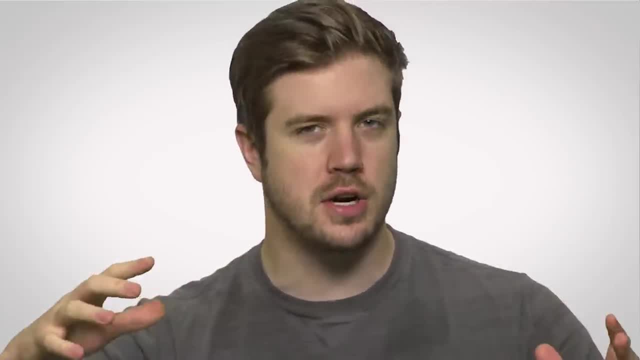 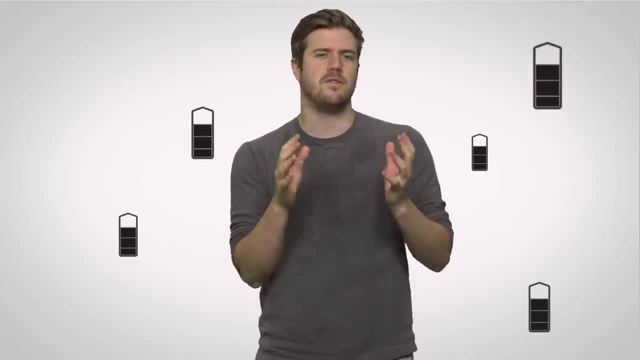 then using a table to track what part of what was stored in each cluster. All right, pretty straightforward and simple. no big deal there. But as hard drives became larger and larger, FAT ran into some problems. Namely, it resulted in a lot of wasted space because it often couldn't fill clusters. 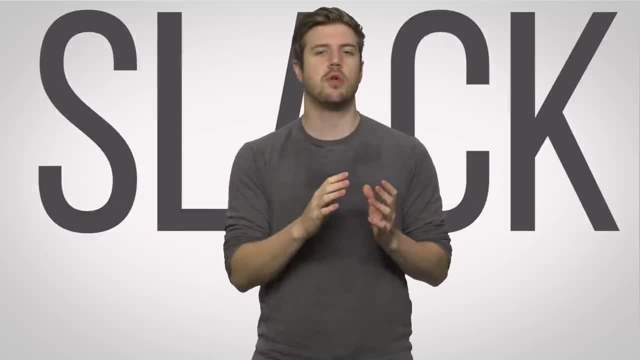 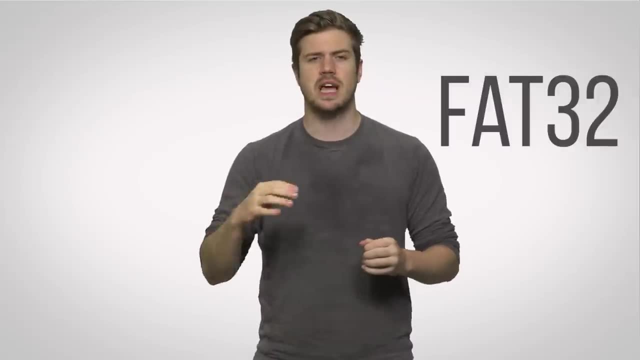 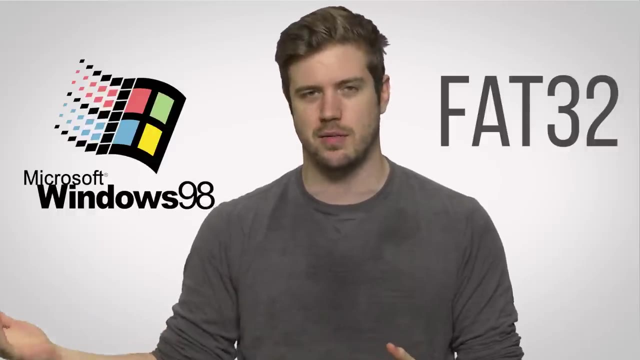 completely a problem called Slack and could only support drives that were kind of smaller due to the way that FAT stored information about file locations. FAT32,, which came to prominence with Windows 98, wasn't an improvement, but still couldn't deal with partitions larger than two terabytes, which isn't 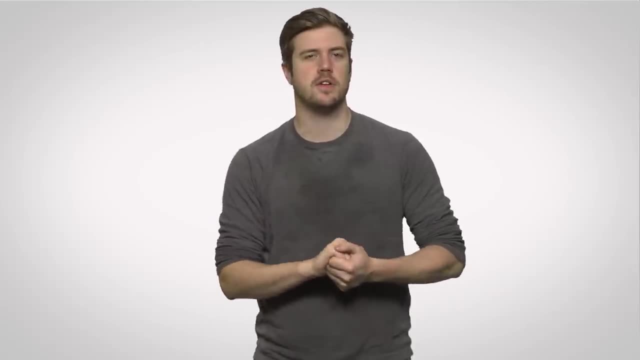 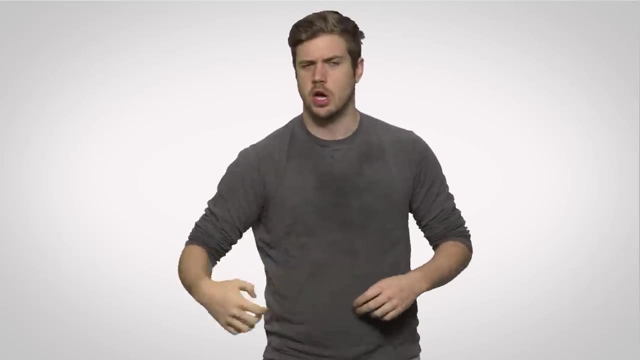 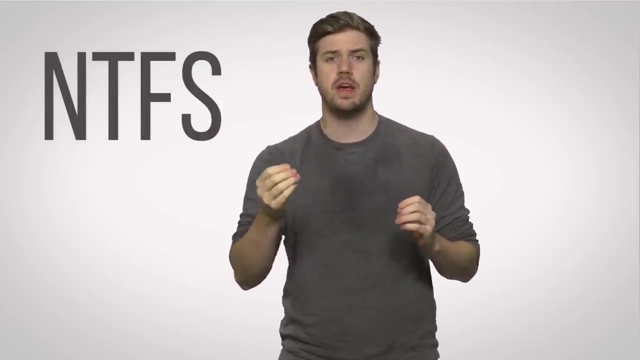 that big these days. To overcome these limitations, every version of Windows since XP and NT 3.1 on the business side of things- has used the only slightly less awkwardly named New Technology File System, or NTFS. NTFS uses some space management tricks to make it use space much more. 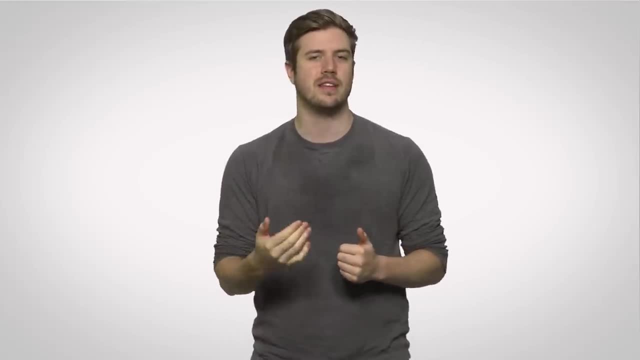 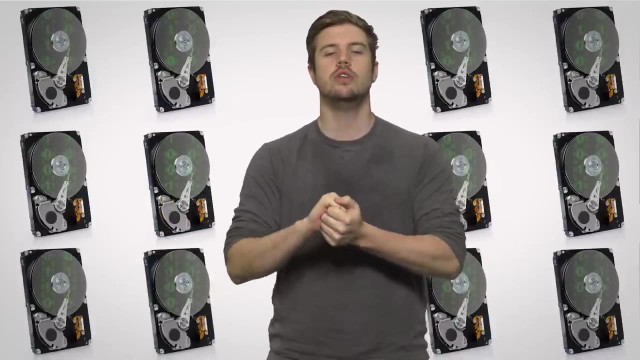 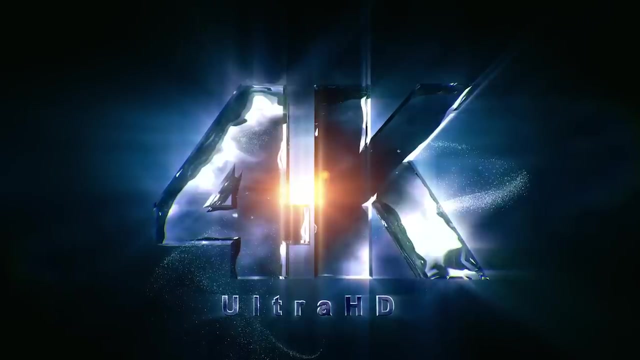 efficiently than FAT, resulting in better real-world capacity in many cases, and can support massive partitions of hundreds of terabytes as well as huge individual file sizes, important in the age of 4K videos that can span multiple hours, making them massive. It also has features to help. 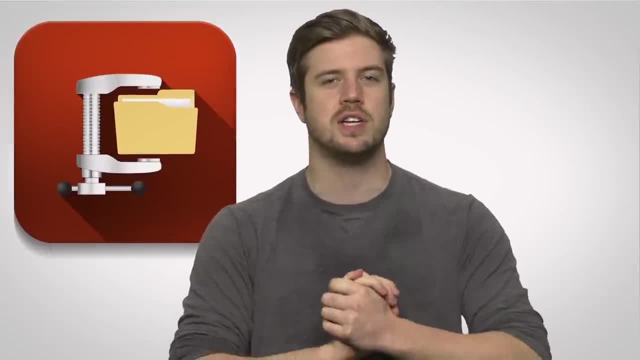 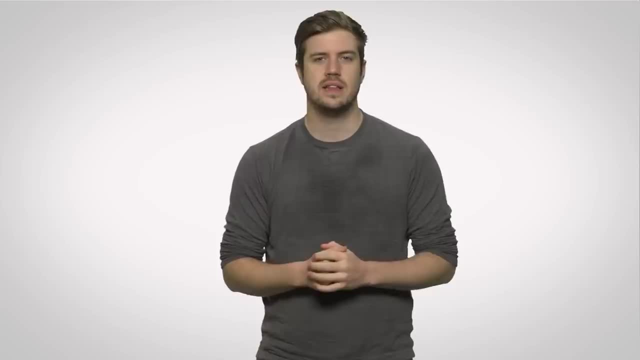 prevent data loss in the event of a crash, native file compression and security features, including native file encryption, support to keep out unauthorized users. These features have made NTFS an almost universal choice for Windows-based PCs these days. But just like it's hard to get rid of those last 10 pounds of fat at the gym, FAT the file system hasn't. 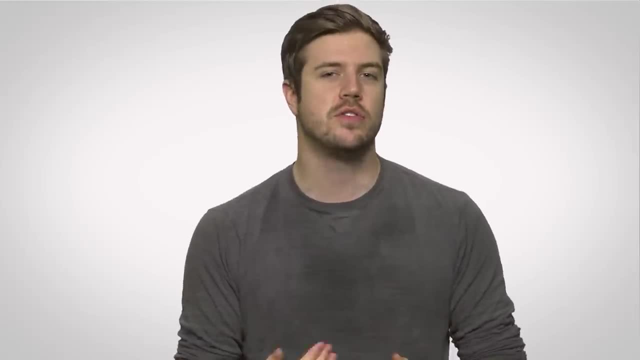 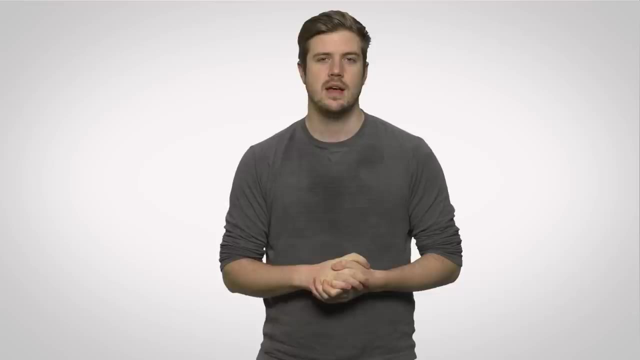 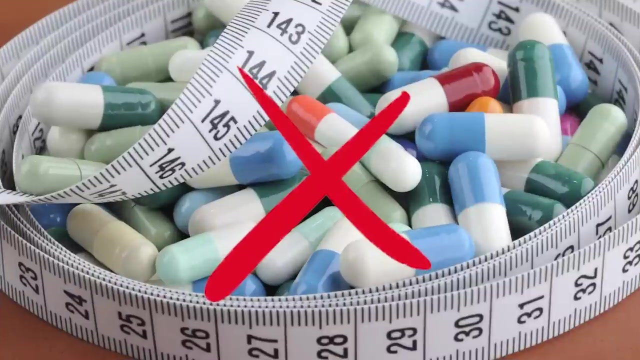 completely gone away. FAT32 is still commonly used on USB flash drives to maintain compatibility with older versions of Windows, as well as operating systems such as Linux. And speaking of flash drives, there's a new version of FAT called XFAT, which is surprisingly not the name of a line of. 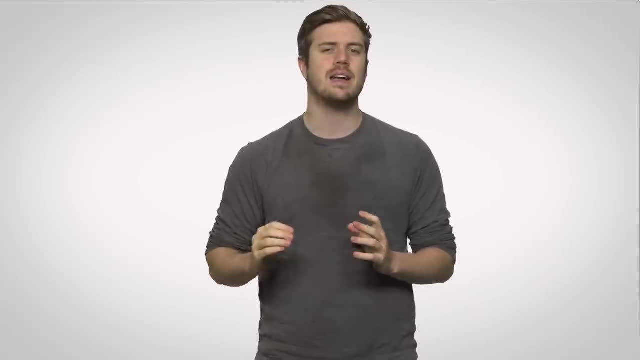 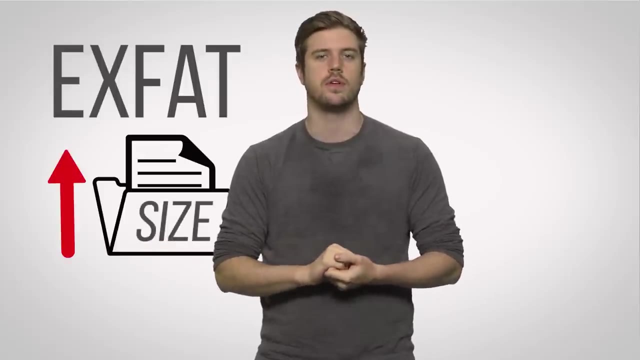 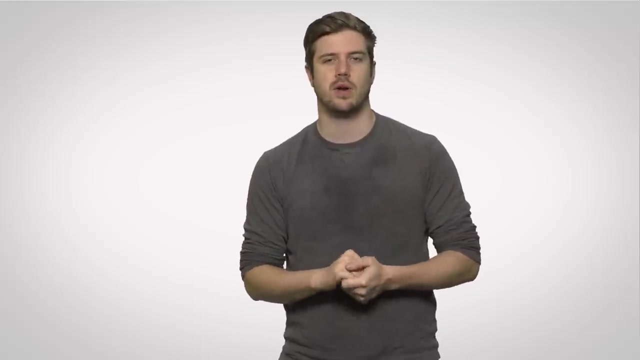 diet supplements. XFAT was designed specifically with high-capacity flash drives and memory cards in mind and support much larger capacities and file sizes than older versions of FAT, while not including features of NTFS that flash drives don't really need in order to keep things running. 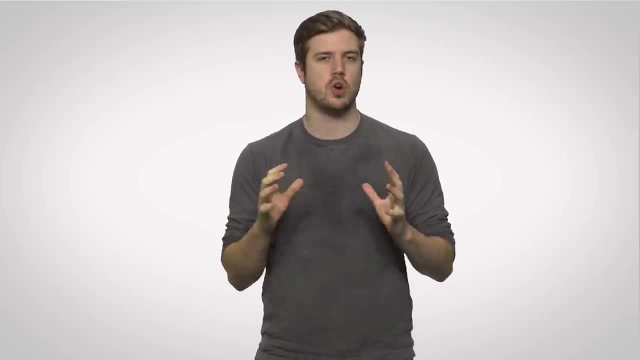 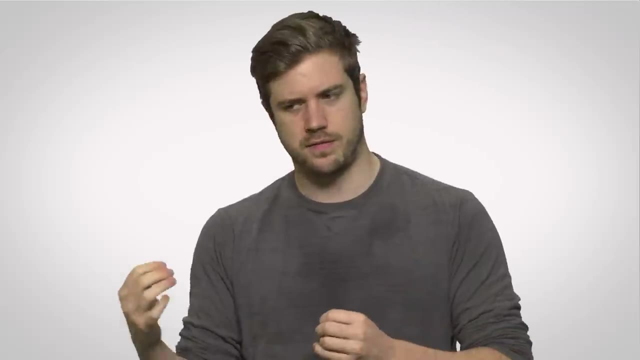 quickly. XFAT isn't always compatible with some quite a bit older versions of Windows, though, so keep that in mind when choosing what you're going to use for your flash drive if you, for some reason, are still using, like, unpatched versions of XP. The good thing, though, is that it's pretty 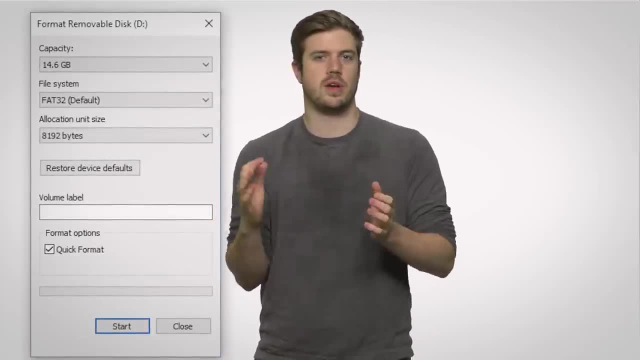 easy to use. So if you're using a flash drive that's not as good as a flash drive. you can switch file systems on your flash drive by just doing a quick reformat After you've saved your file somewhere else. of course I don't want to be responsible for that, But no matter what you. 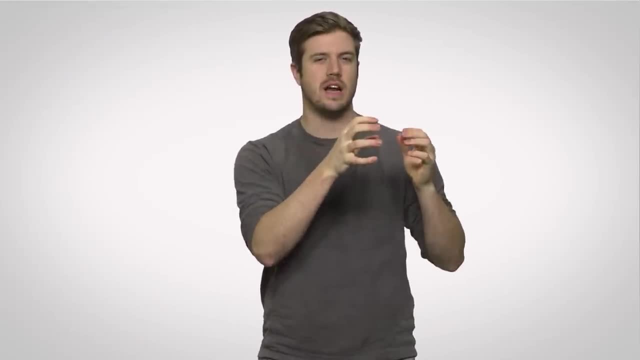 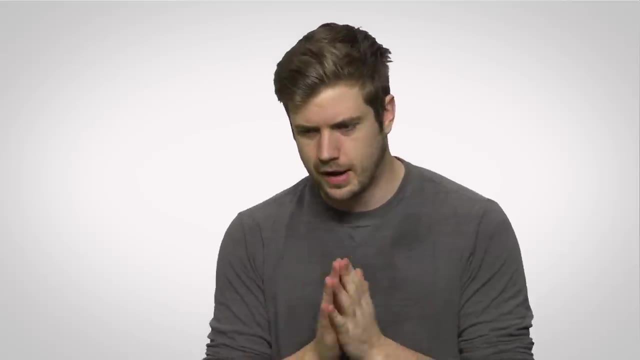 choose. you can bet that your drives will keep track of your data better than your roommate, who is always asking you where the TV remote is. Are you ready for a Linus-style segue? I got this one. I got this one. Speaking of keeping track of things. keep track of your education with 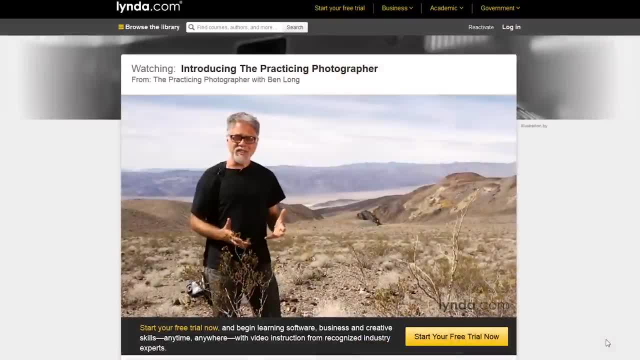 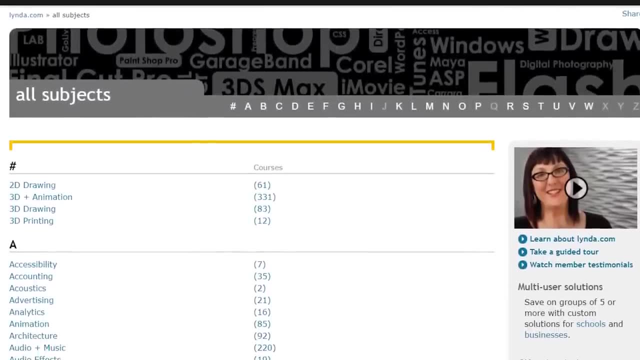 lyndacom. With a lyndacom membership, you can watch and learn from top experts who are passionate about teaching. You can stream thousands of video courses on demand and learn on your own schedule at your own pace. You can browse each course's transcript to follow along or to. 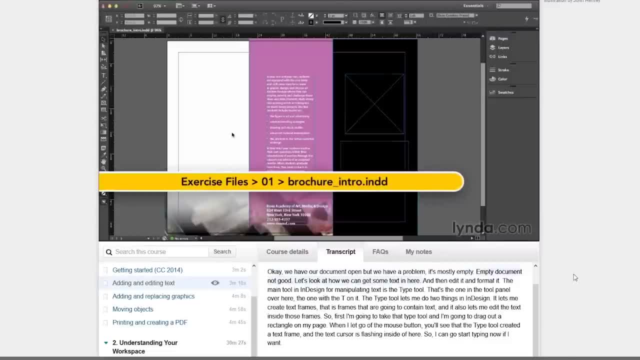 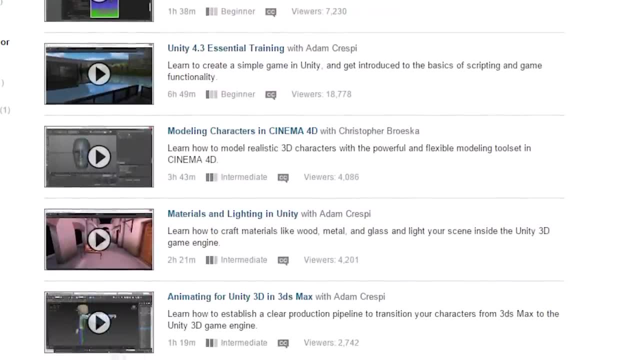 search for a specific keyword that you may have missed and skip to that point in the video, which is actually super helpful. You can take notes as you go along and refer to them later. You can download tutorials to watch them on the go. You can access it on iOS, Android, PC, basically whatever.